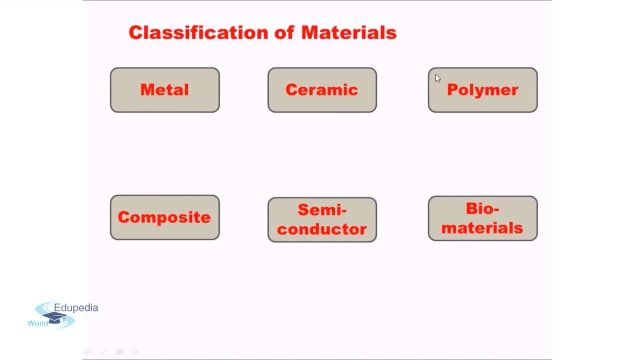 and biomaterials. so the initial four of them, the metal, ceramic, polymer and composite, are the most broad categorization of the materials. semiconductor kind of fits into this scope. so are the biomaterials. so basically these things are a subgroup, let's say, but mainly we have what is known as metal, ceramic, polymer, composite. 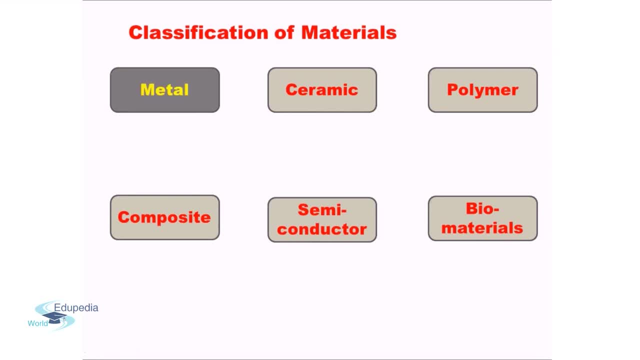 now let us pick each of them one by one and see. to begin with metals. the most prominent property of metal is that the electrons in a metal are non-localized. that is when we will discuss about the atomic arrangement of electrons, protons and neutrons. we'll see that the metals have what 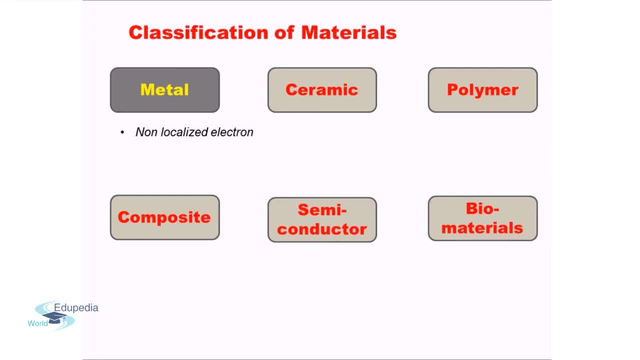 is known as non-localized electrons. and the electrons in the metal are also non-localized, and that is the outer valence. electrons do not belong to individual atom, rather it belongs to the whole bulk of the material. and this non-localized electron kind of gives the properties to the 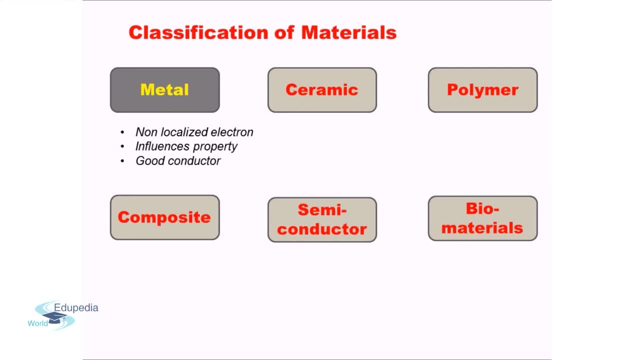 material so influences the properties. then we have what is known as good conductor. since there is non-localized electron, those electrons are free to carry charge, thereby conduct electricity. that is a trademark property of metals. metals normally have a lustrous appearance, that is, they are more on the shiny side. these four are very basic properties. there are many more properties. 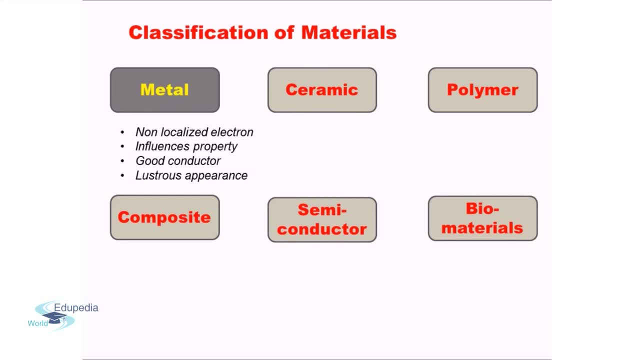 of metals, which we will explore in details in further chapters. but to give you a taste, these are kind of the properties. then ceramics: ceramics are mainly oxides, nitrites and carbides. so if you have some oxide, zirconium, diboride, borides are also. 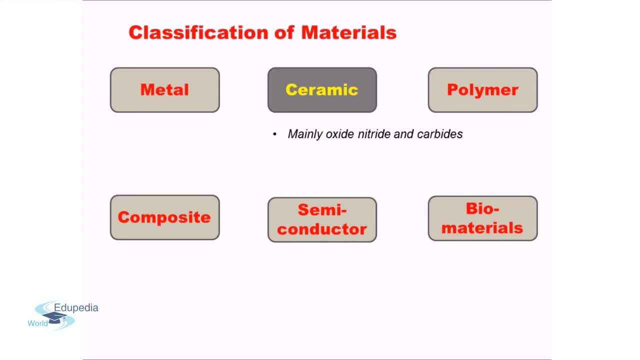 ceramics or carbide. those things are fall under the ceramic category. then we have insulating properties, so ceramics are normally non-conductors or they are very good insulators. thereby a lot of application of ceramic is in the field where there need to be insulation from electricity or 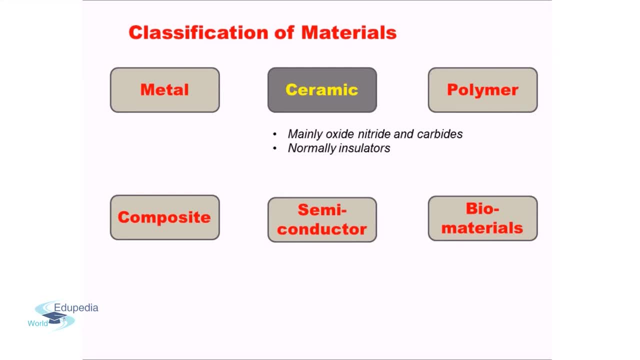 insulation from heat, but there is also extremely important conducting properties under different circumstances, and those things we will see in details later. ceramics are hard and brittle. they have a very high hardness and they break easily. that is, if you drop a ceramic material, the chances are high that it will break immediately. next up, let's discuss about polymers. polymers are mainly 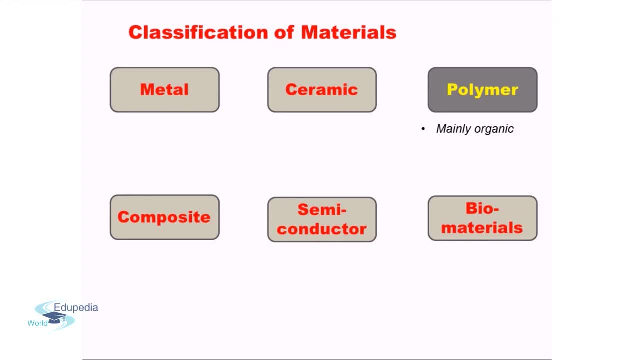 made up of organic molecules. some of the examples of polymer can be rubber and plastic today, examples which you encounter every day. but the extent to which polymers are being used is much, much more broader than just rubber and plastic. polymers are normally very large change molecules. 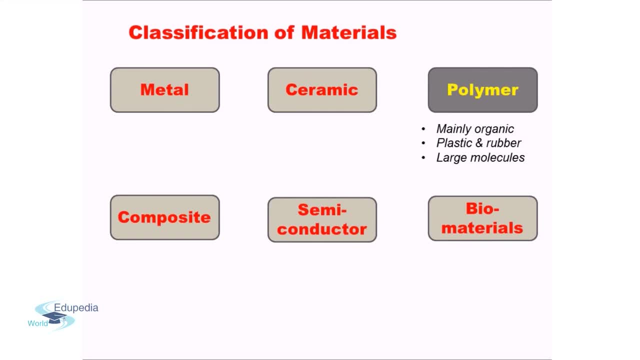 that is, the molecules are not small molecules. they are quite large and that makes the molecules bulky. they have a very high molecular weight and polymers are normally low density materials, that is, they are not compactly packed. thereby their density is low. and polymers, mostly, are flexible materials. need. 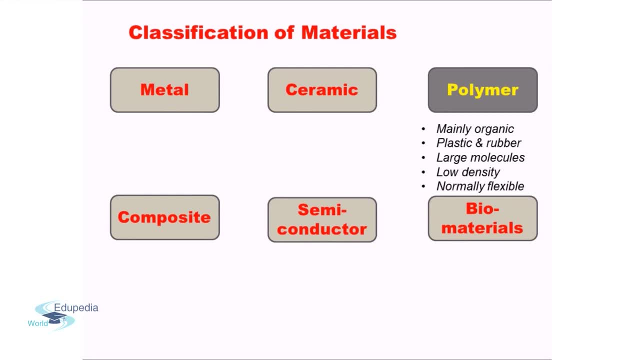 not be the case always, but generally speaking, they are on the flexible side compared to ceramics materials or metals. let's let us see what are composite materials. till now, what we have seen is that all the three- metals, ceramics and polymers- are made out of one type of material. right, but composites are made of more than one material. 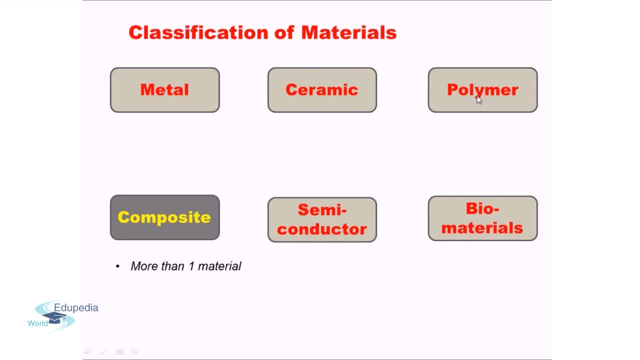 they might have two metals, let's say. or they might have a metal and a ceramic, let's say. they might have a metal and polymer, or any combination thereof. it may have more than two material too. now what is the reason of using more than one material? suppose you have one. 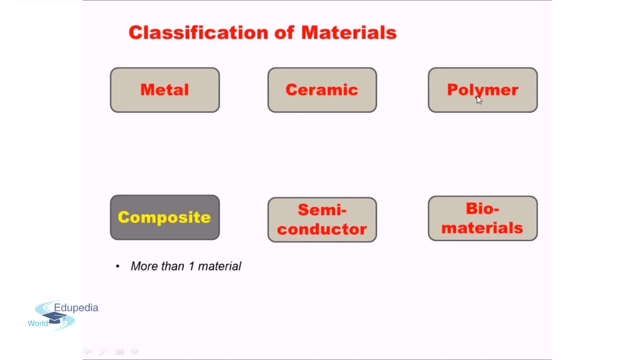 material which has very high strength and you have another material which is very high strength, which is also a very high material, which is quite flexible. but the first material is not flexible and second material is does not have a high strength. so what you can do is you can combine. 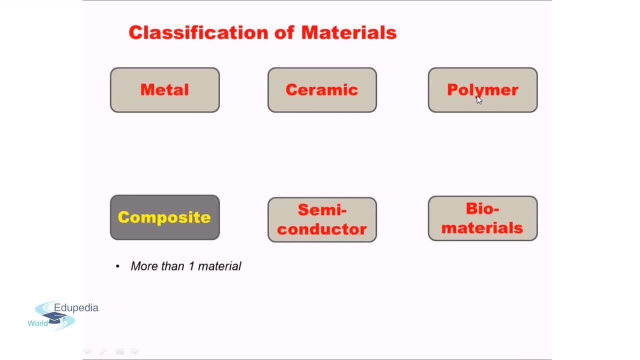 the two materials and get a moderately good flexibility while retaining a moderately good strength. so, depending on the application, you can find combinations of materials which gives you the relevant properties you need for the application. that is the power that composite material provides us with. basically, composite materials provide best property of constituent material and one simple. 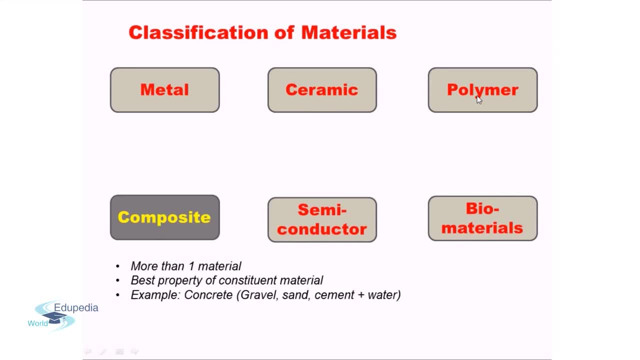 example, is concrete that is used for house building, that has gravel, sand, cement and water. so there are different materials, you see, and those. each material brings a inherent property with itself and they combine together to give our required application. that is the binding property of the whole concrete system. so now we have seen the four broad classifications of materials. let 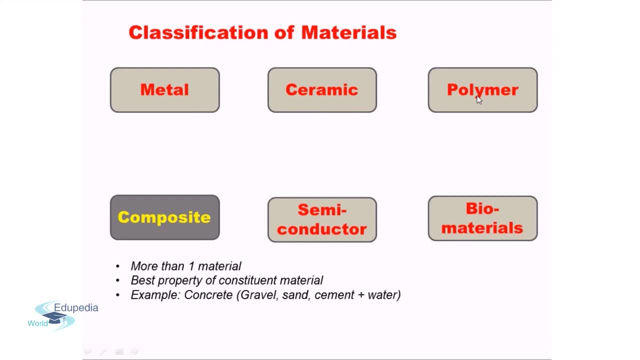 us jump into the two kind of subcategories of material. one is semiconductor, as the name suggests and as you might have studied in your previous classes. a semiconductor is a material which has intermediate conductivity, that is, they are not as good a conductor as metals, but they not a insulator. and this semi conductivity of the material has interesting applications. 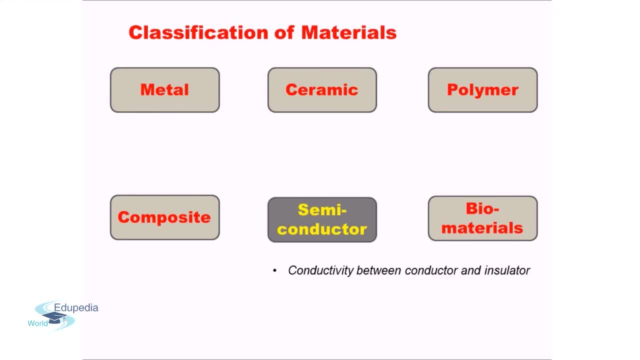 specially in the integrated chip system or the electronic area. you need to control the amount of conduction that takes place, and semiconductors give you precisely that control. how can you control a material which is a semiconductor- let's say, for example, silicon has a certain conductivity- but by something, what is known as doping, that is, adding different? 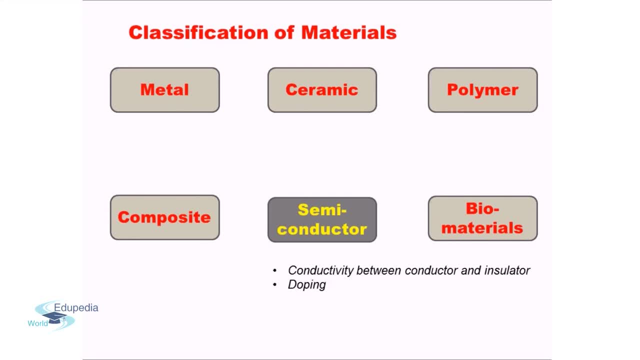 element to the silicon base in very controlled amount can help you fine tune the amount of conductivity you want to provide in the material. so semiconductors are basically very good at adjusting the amount of conductivity based on the amount of additional element you dope into that material. 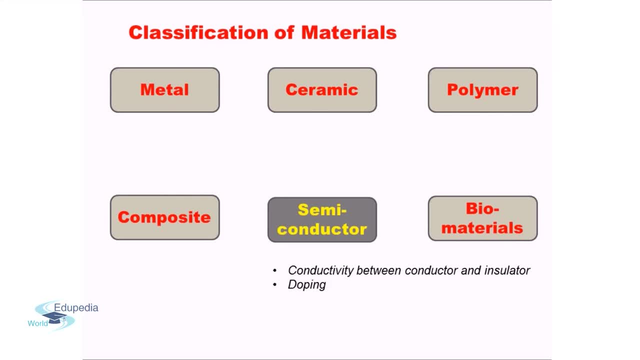 that gives you a fine tuned way to control conductivity, and obviously this has brought about the integrated chip revolution, which is kind of the modern revolution, in the sense that all the electronic gadgets you see today is due to this semiconductor industry. finally, let us discuss briefly about biomaterials. now, what are biomaterials? exact definition. 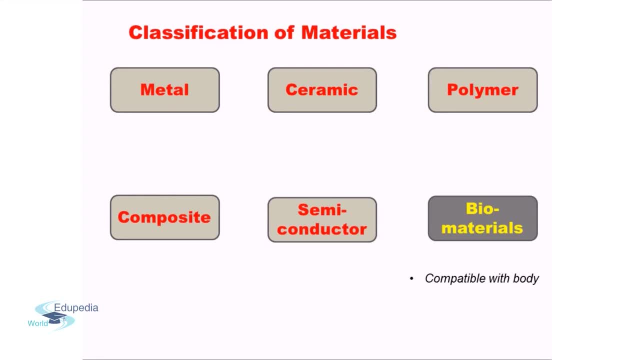 is that these are materials which are compatible with body, mainly, in our case, with the human body. let's say, there is a need for knee surgery, replacement of the knee or the hip bone. so when you are inserting something into the body, like the hip joint, that new material introduced to the body should be biocompatible, or it should. 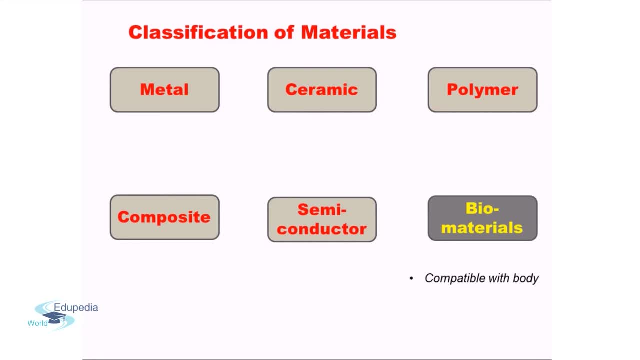 be compatible with your body. else it will degrade inside the body and that will lead to a very tragic condition inside the body which can eventually lead to even death. so such materials which is compatible with the body and which can be placed inside the body safely are known as biomaterials. this has 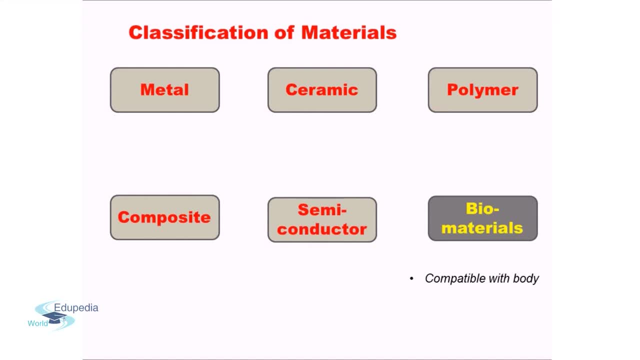 a wide application, as you can think, in the medical area, mainly used, as in implants. as I explained and speaking about it, the it can be any of the above five, or mainly the four categories, for example, ceramic, polymer or composite, not necessarily a semiconductor, because this itself 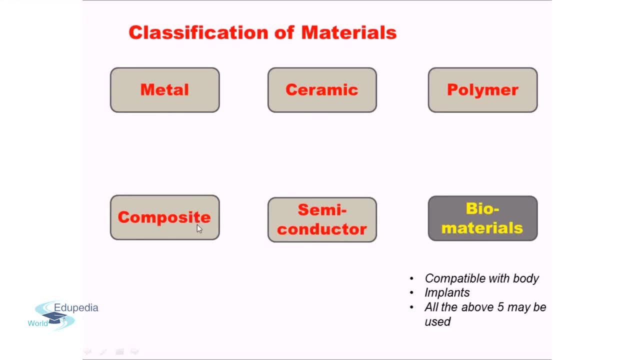 falls under a combination of these categories, right? so this gives you a broad picture about what are the different kinds of materials and what can we expect from this course at large. specifically speaking, this particular introductory course will mainly focus on metals and metal alloys. we have discussions on ceramics, composite and polymer too, because they are interesting. 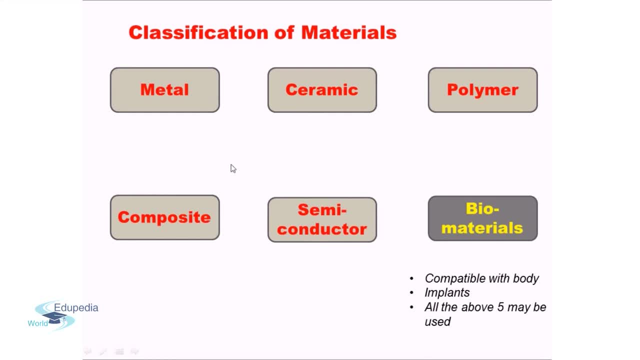 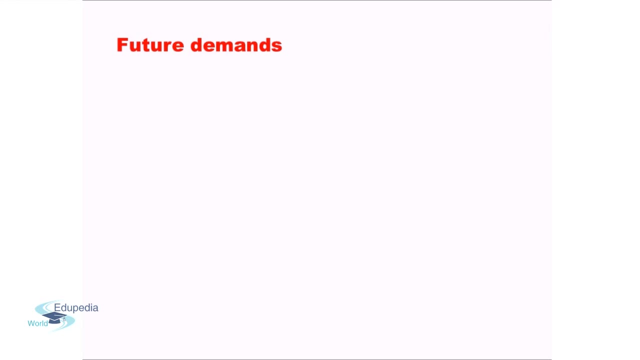 topics, but they in themselves are much, much wider topics and complete courses can be offered on each of them individually. with this classification, let's see what are the future demands in the area of material science and engineering. till now, what we have seen. we have seen the history about material. 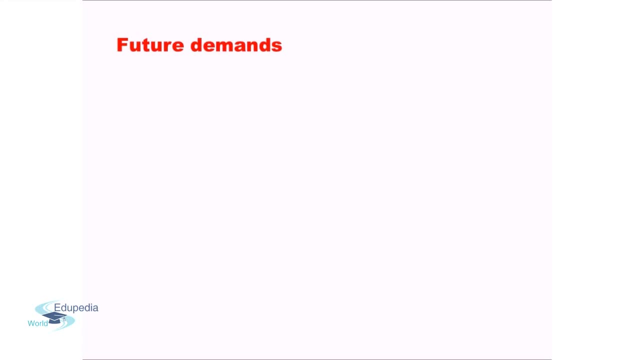 science and engineering. how did it come about into being? what are the present applications of it? and then we saw different kinds of material. now, what is the future of it? one very simple thing which you can think on your own self is that sophisticated materials while maintaining the environment. 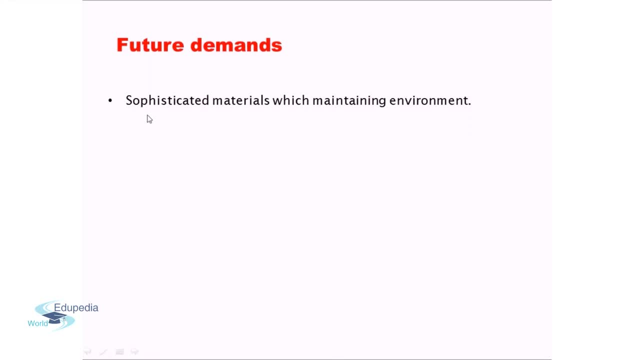 what do I mean by this? we need to keep on coming with new materials. with ever increasing demand of new applications, ever increasing demand in terms of strength or particular electrical application or magnetic application, we need to keep coming up with new and better materials. so that is what sophisticated. 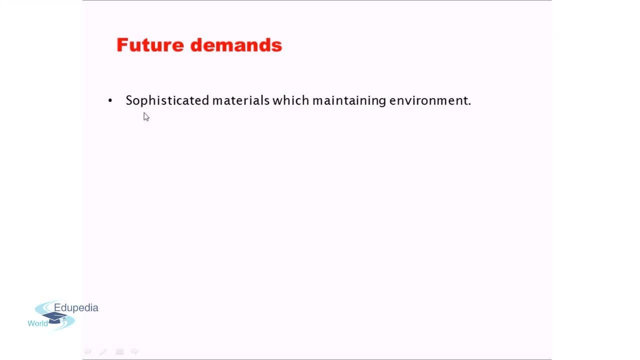 material means and maintaining environment. global climate change is a very important thing that needs to be taken into consideration, and we need to work towards maintaining the environment while making our own life better. so we need to create the materials in such a way that the materials in itself do not harm the 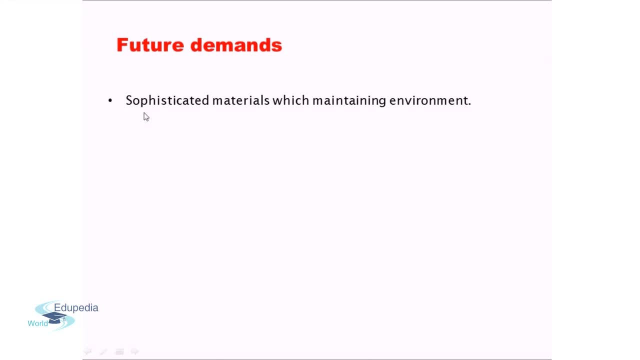 environment or, while manufacturing the material, the environment is harmed as less as possible. next, the nuclear revolution needs new materials. what is the nuclear revolution? till date, our source of energy is mainly from the coal industry. there are renewable sources for energy being generated and used of late. 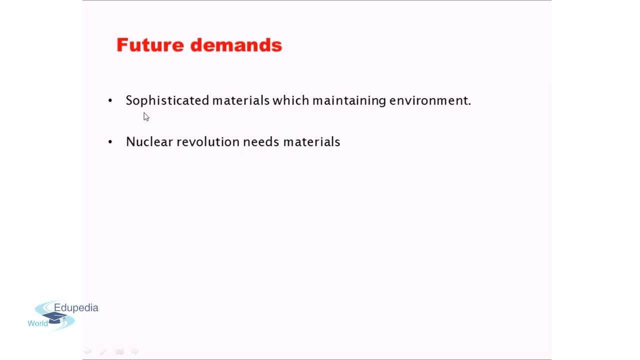 with knowledge about how much harm coal does to the environment, burning coal and stuff- but still one of the most important area which is not yet tabbed into is the nuclear regime. it is being used, but not to its full extent, so the nuclear revolution needs to take place. that 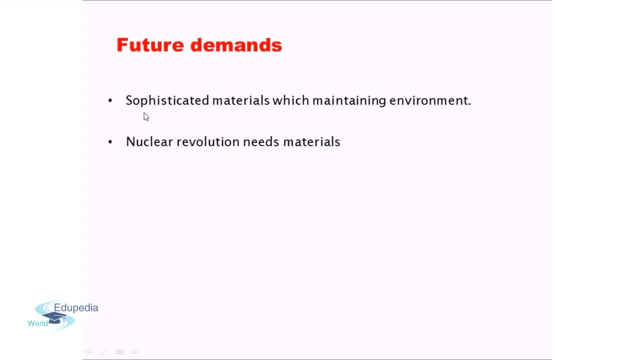 is the source of infinitely large amount of energy, but it is still not used. but it's a very risky deal. so new and sophisticated materials which can withstand very harsh conditions and which can protect us from nuclear radiations, such things needs to be come up with. so that is a challenging field which is one of the futures of material science. 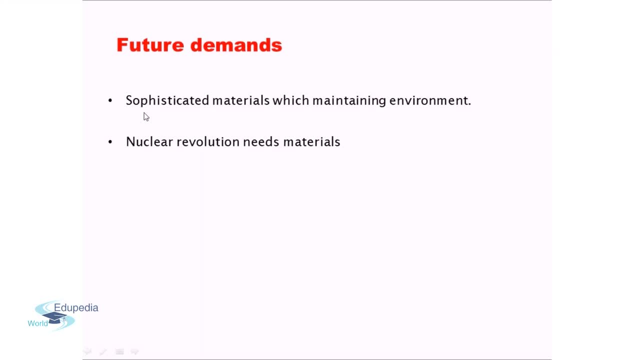 and engineering, you need to bring about ingenious, noble ideas to deal with this problem. then the transportation sector- the whole transportation sector- is a game where you are trying to reduce the weight, thereby increasing the efficiency of the vehicles. that is one of the most important research area. therefore, weight reduction is one of the most prominent ideas that we need to be. 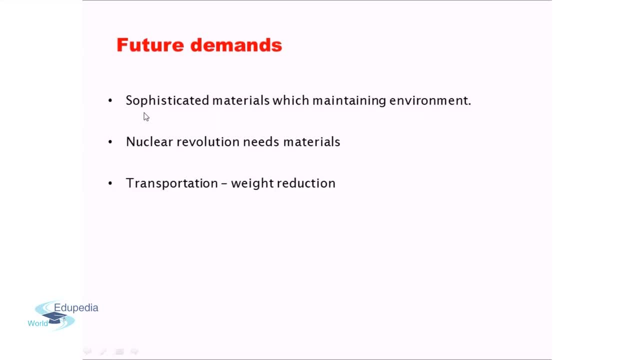 working on and in fact a lot of research is going on in that field. so this is actually a very well known field which is already being ex explored in the원 paris Aircraft Trust problem solving into, but which has a lot of future prospect to solar technology, as i mentioned about the energy. 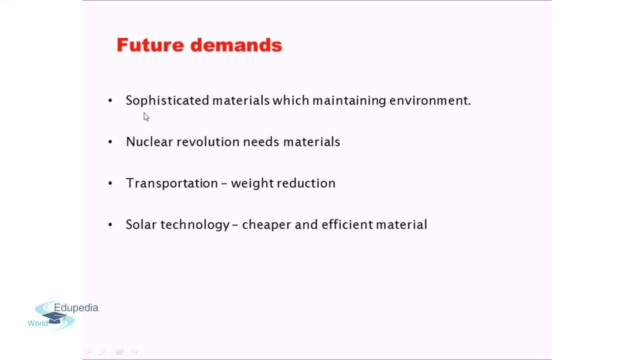 we keep coming back to energy. why? because that is a direct relevance with the climate change. so, coming to solar technology, solar technology is already being put to use. there are a lot of things that are running on day-to-day scale using the solar technology, but do you know what is the? 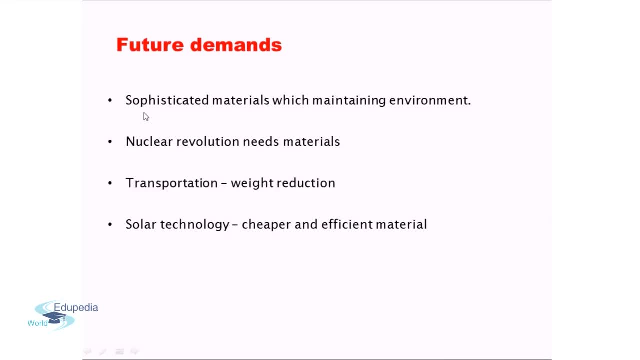 main problem with solar technology? the main problem is that the efficiency of the materials which we have at present to capture the solar radiations is very low. it's in the range of around 20 percent. so we are actually not utilizing the solar energy as much as we can. we need to find 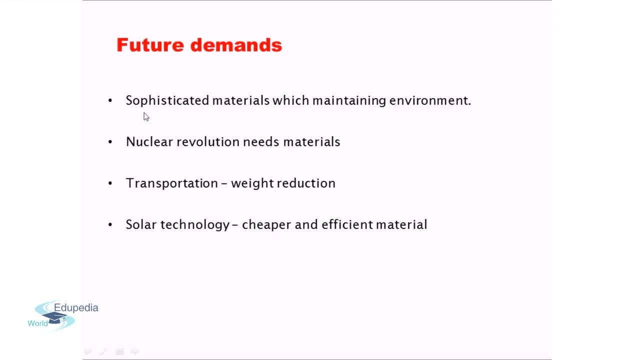 new materials and new ways to harness the efficiency much higher than 20 percent, or even a little higher than 20 percent. that is also going to give a lot of increase in the energy input through the solar technologies. work needs to be done in that field. then, coming back to the metals, 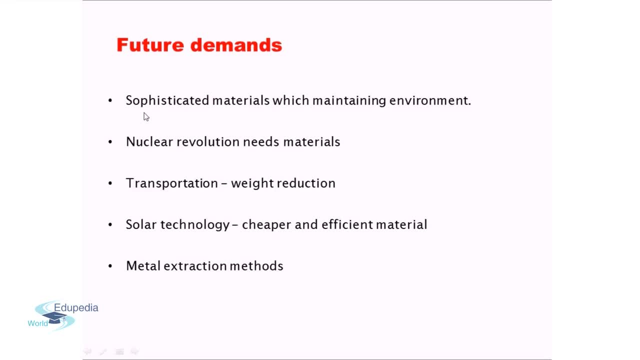 point, metal extraction methods. metals normally, except for the noble metals, do not lie around in the earth's crust right. you need to dig out the ore and then put it through extraction processes and then the metal is obtained from it. but this is a highly energy intensive property. a lot of